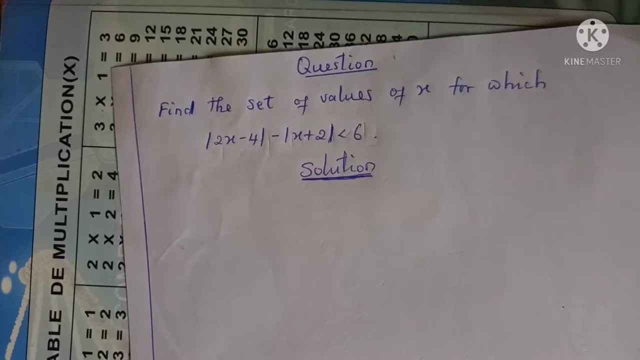 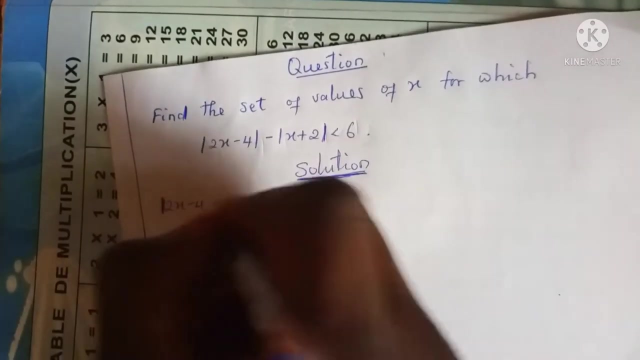 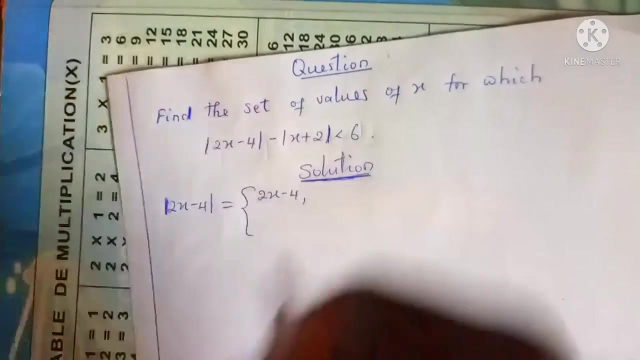 And to solve this in-equation, I will start by defining the two absolute value functions in this in-equation. So I will start by defining the absolute value of 2x minus 4, and we know that the absolute value of 2x minus 4 is equal to just 2x minus 4 if 2x minus 4 is greater than or equal to 0, or if x is greater than or equal to 0.. 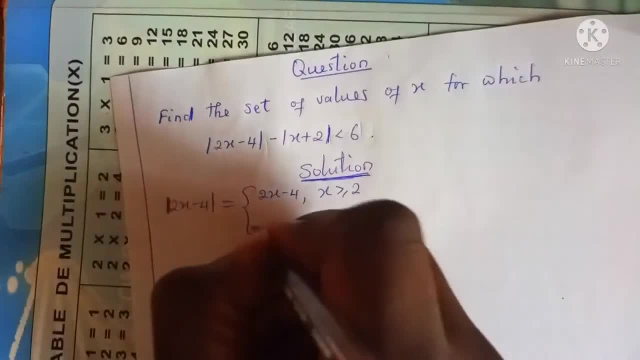 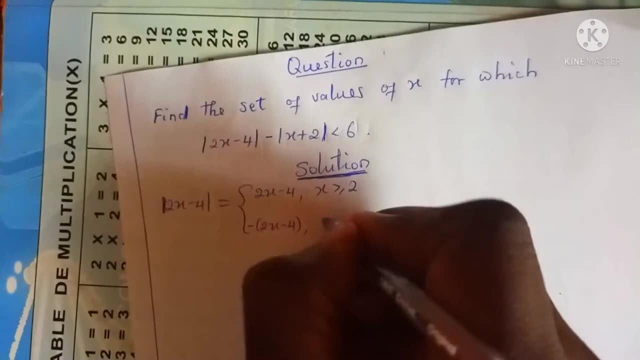 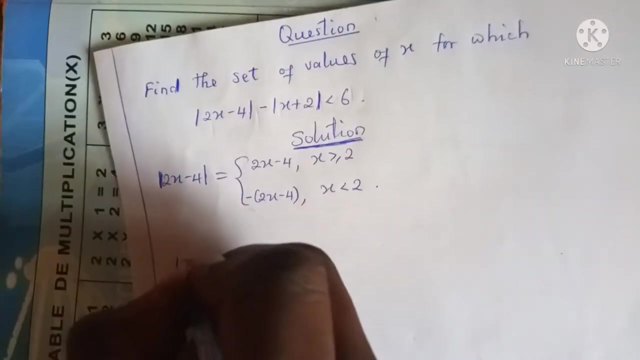 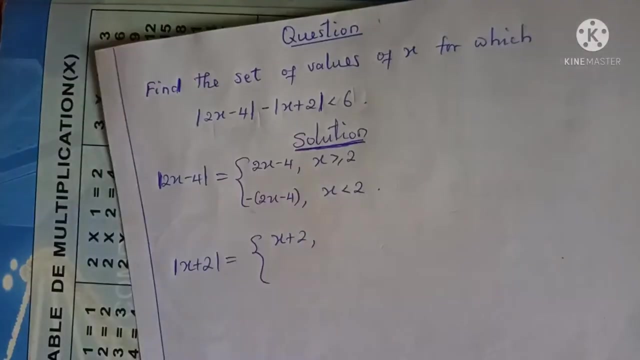 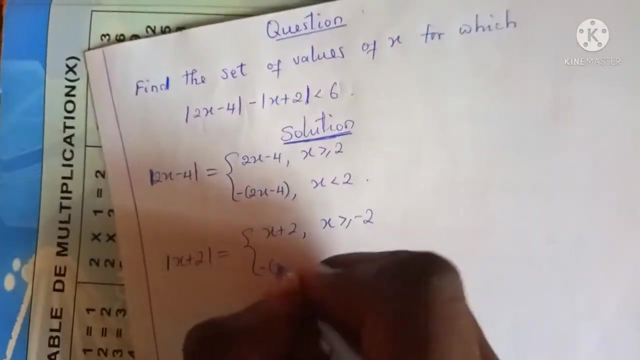 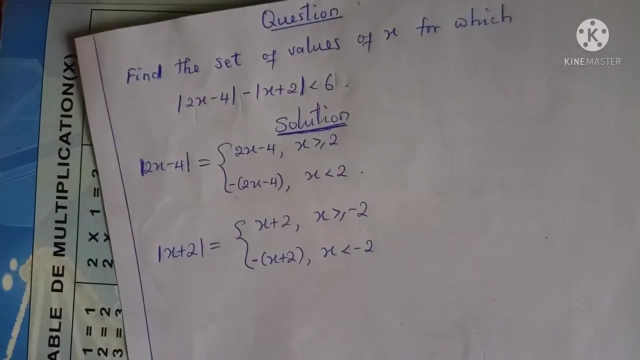 And I will also define the absolute value of x plus 2, which is just x plus 2 if x plus 2 is greater than or equal to 0. or if x is greater than or equal to negative 2.. Or negative into x plus 2 if x plus 2 is less than 0 or if x is less than negative 2.. 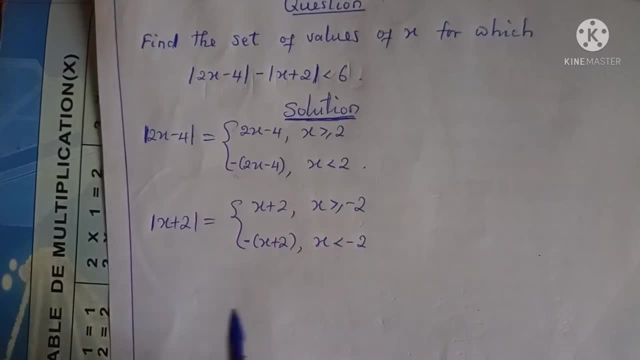 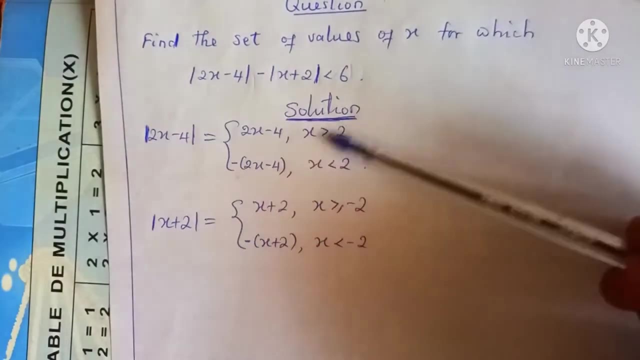 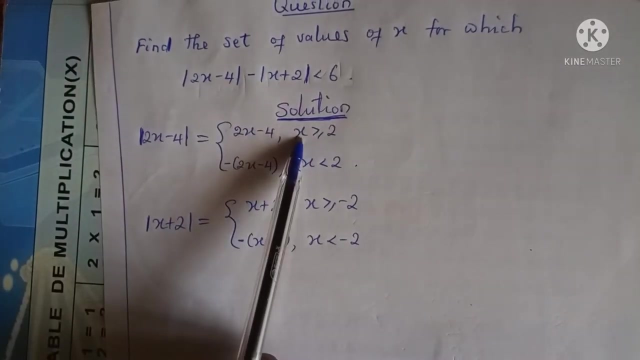 Now, at this level, I am going to find the intersection of this interverse. I will look for the intersection of this pair of interverse here. Now, when you look at this first, two interverse x greater than or equal to 2 and x greater than or equal to 0. 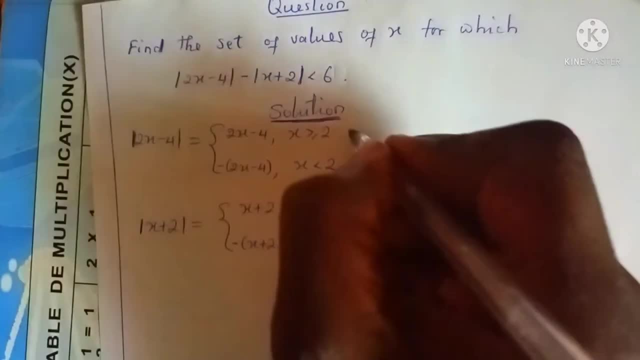 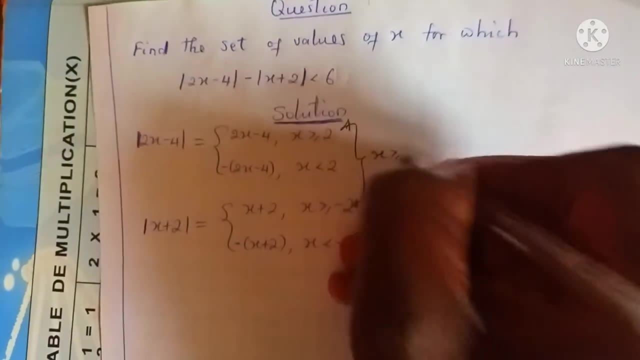 When you look at this first two interverse- x greater than or equal to 0 and x greater than or equal to negative 2, we can easily get the intersection, which is the set. I am looking at these two branches. the intersection is just the set x greater than or equal to 2.. 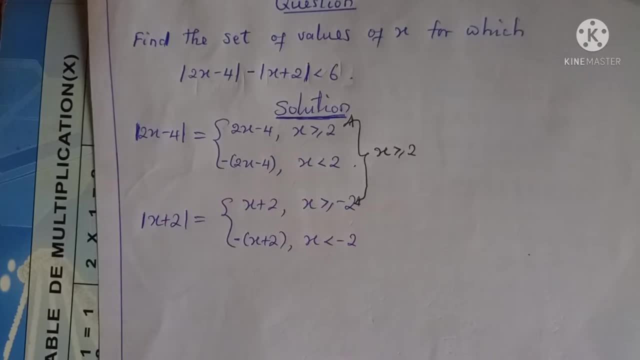 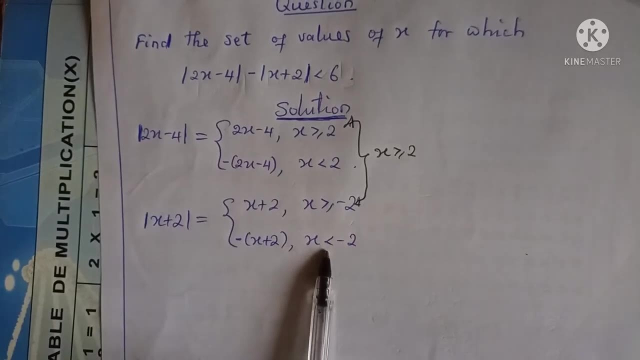 You can get this intersection easily by using a normal line. If you take the first branch here and the last branch here, you discover that the intersection is an empty set, because you cannot find a value which is greater than or equal to 2 and at the same time less than or equal to negative 2.. 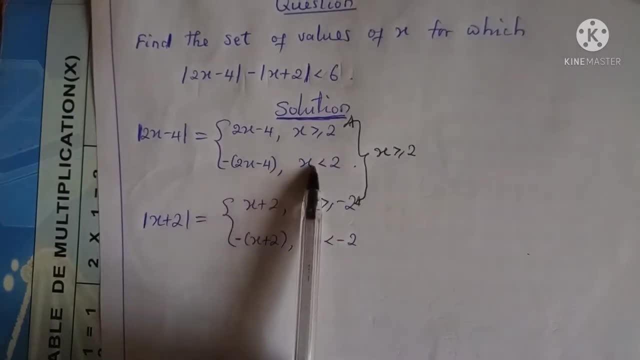 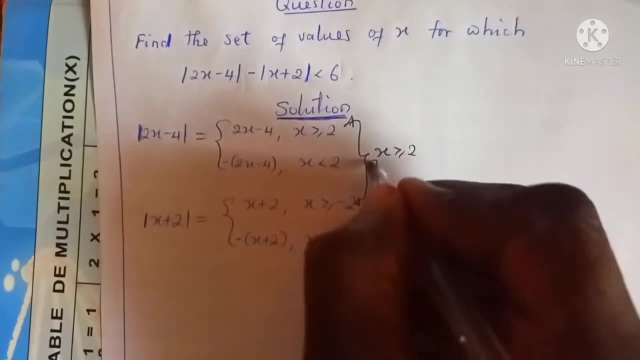 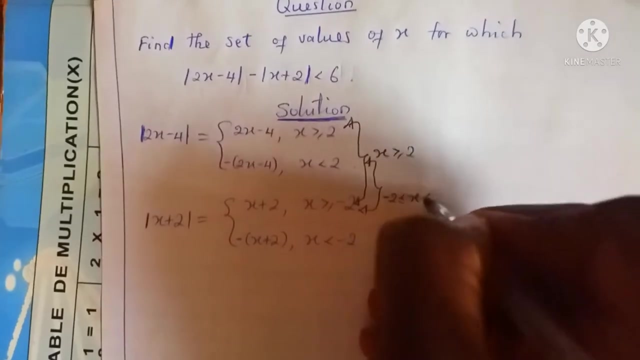 Now let's look at these two branches, that is, x less than 2 and x greater than or equal to negative 2.. What do you think will be the intersection? The intersection at this level will just be the set, the interval: negative 2 less than or equal to x which is less than 2.. 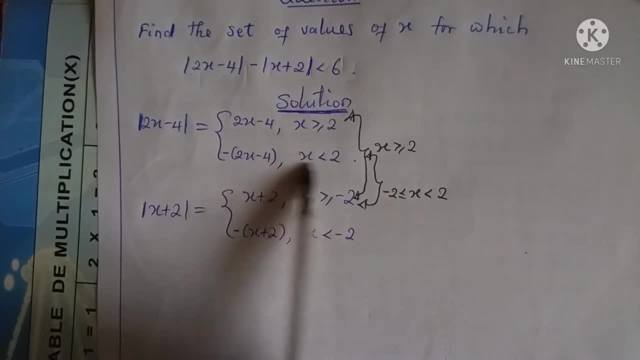 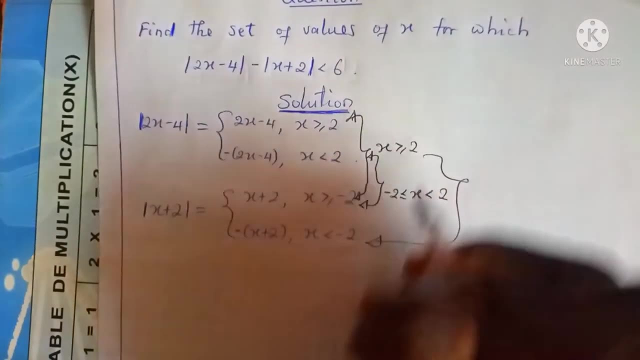 And then the last branch. we are going to look at this and this And if you get the intersection of these two, you will get the intersection of these two. These two, You are going to obtain the set x less than negative 2.. 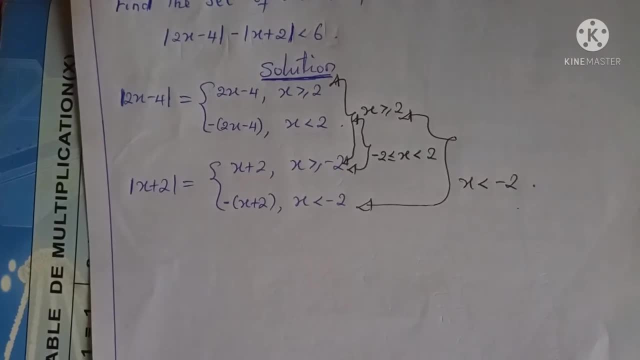 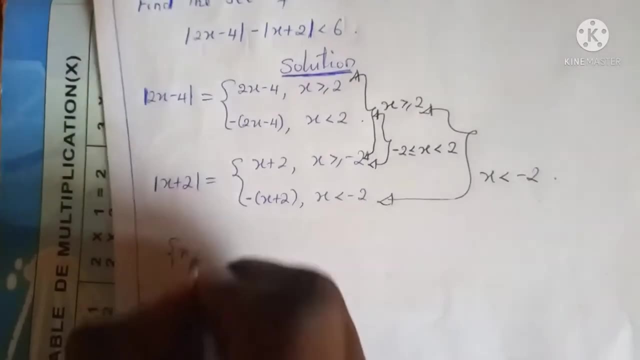 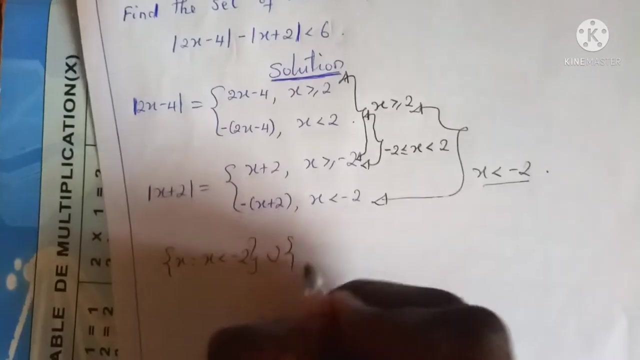 Good, At this level, you can partition the set of real numbers into three. This is what we are going to obtain, That is, if you take the set x, such that x is less than negative 2, this one union the set x such that negative 2 is less than or equal to x which is less than 2,. 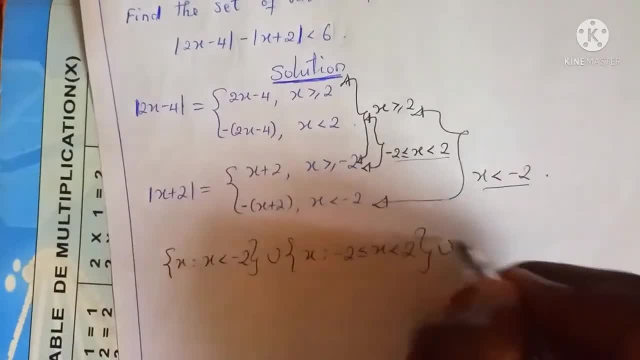 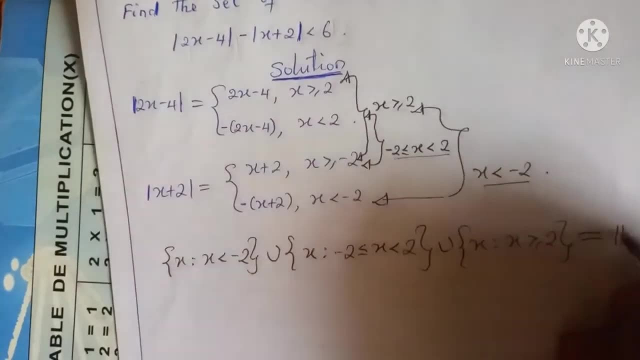 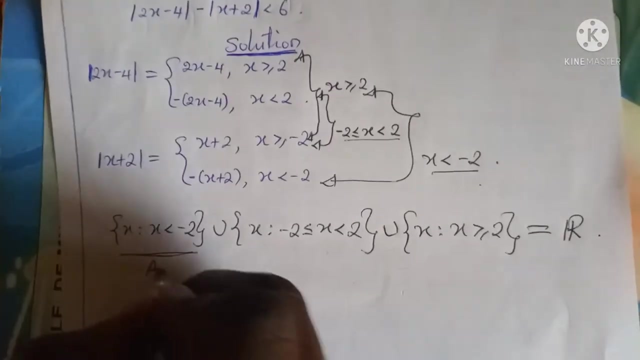 that is, this one union, the set x, such that x is greater than or equal to 2, we are going to obtain the set of real numbers. Good, Now let's call this set A, call this one B and call this one C. 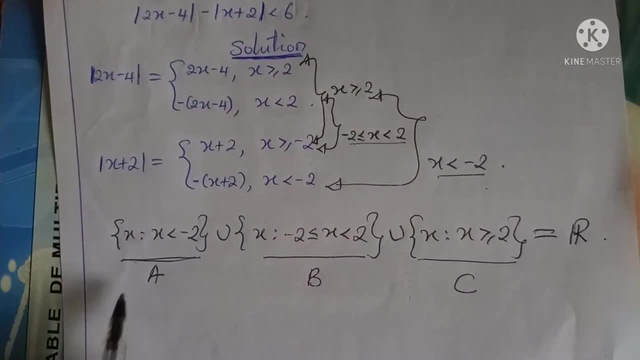 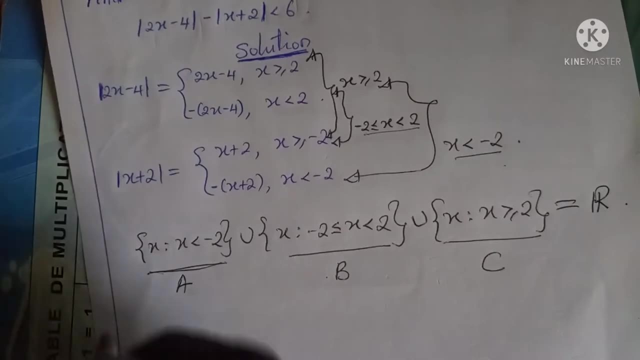 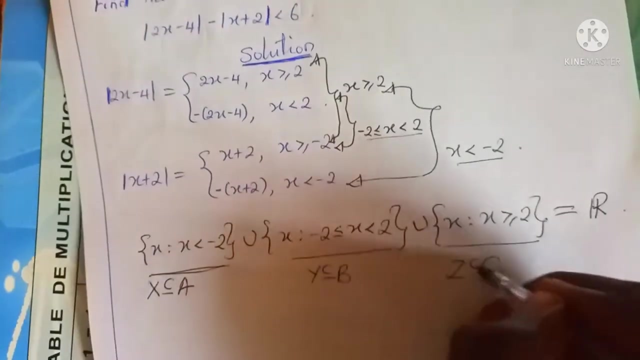 So we are going to find the subset of A, the subset of B and the subset of C which satisfy this given in-equation. Let's call that subset of A x, the subset of B, y and that of C. let's call it z. 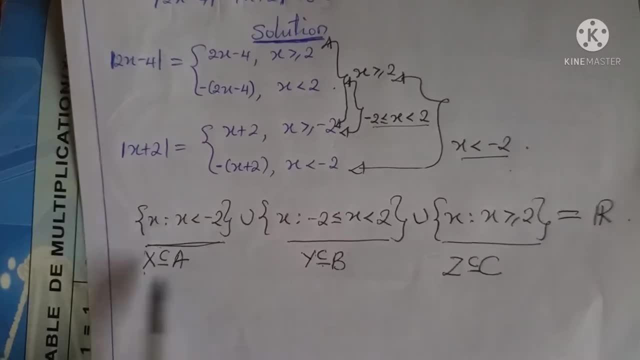 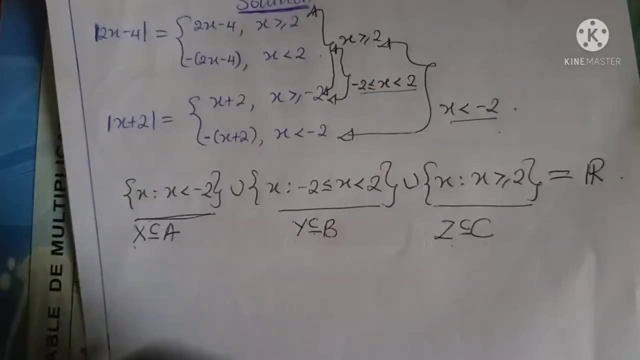 So at the end, if you find x, y and z, we are going to obtain the solution of this in-equation by taking the union of these three sets, that is, x, y and z. So how do we find x? 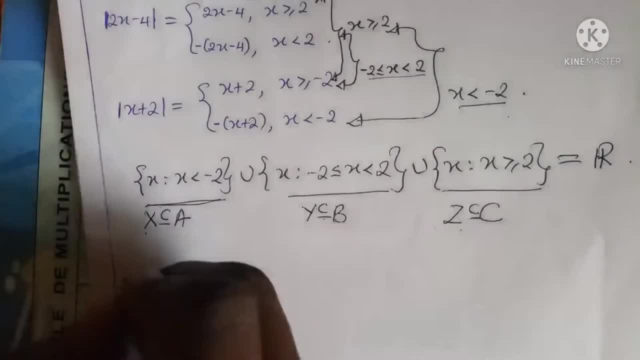 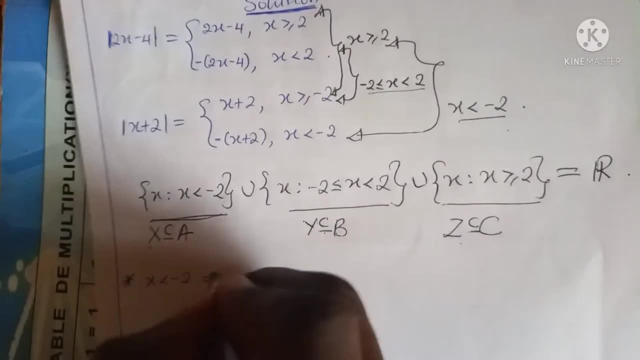 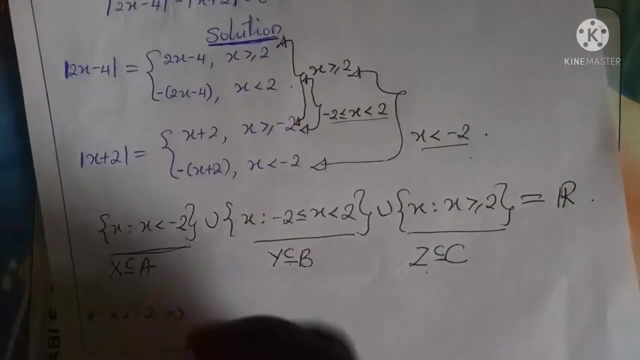 To find x. we are going to start with the set A, And A says that x is less than negative 2.. And we know if x is less than negative 2, look at these two branches. if x is less than negative 2, then the absolute value of 2x minus 4,. 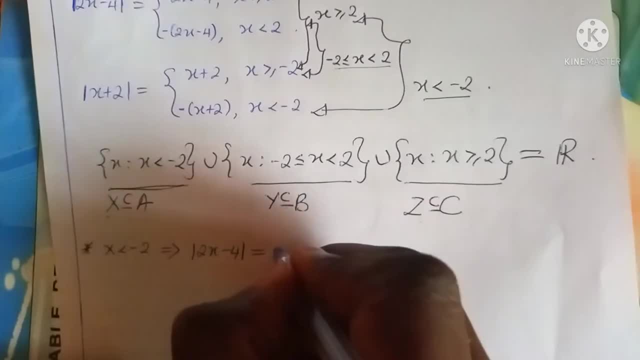 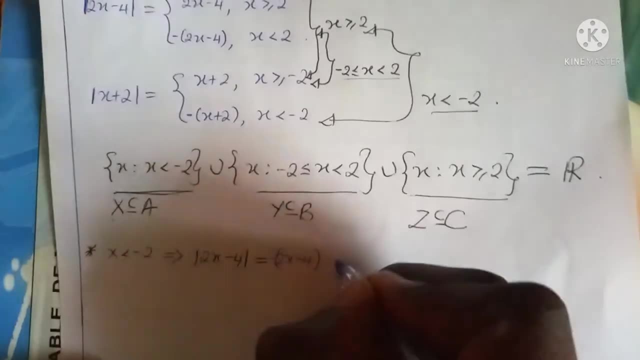 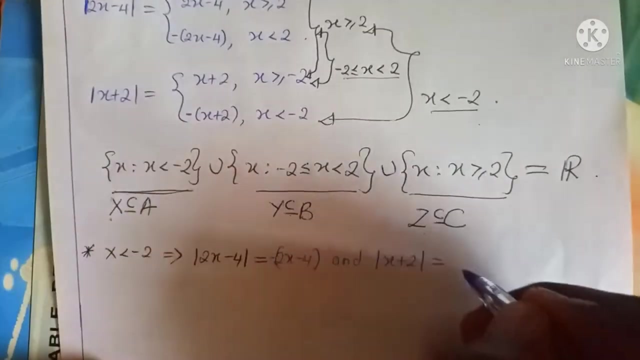 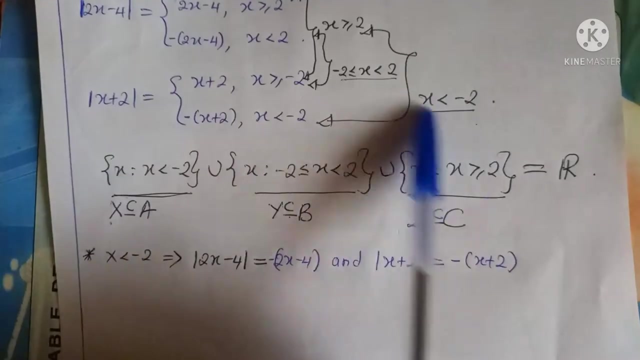 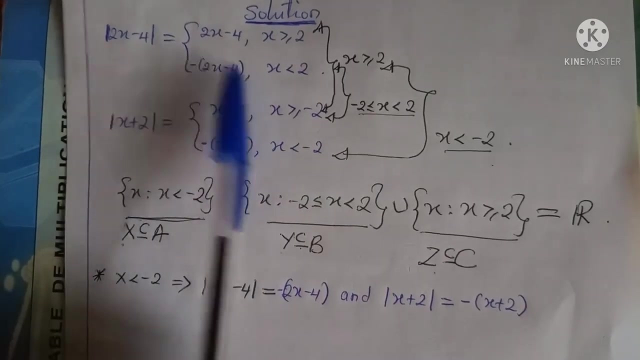 the absolute value of 2x minus 4 will be negative into 2x minus 4.. And the absolute value of x plus 2 will be negative into x plus 2.. Yes, from this interval, You know, if x is less than negative 2, the absolute value of 2x minus 4 will be equal to negative into 2x minus 4.. 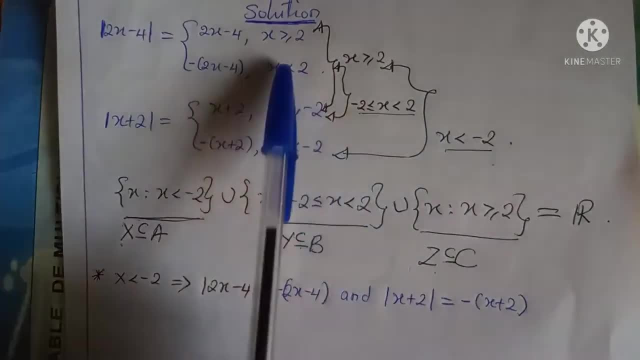 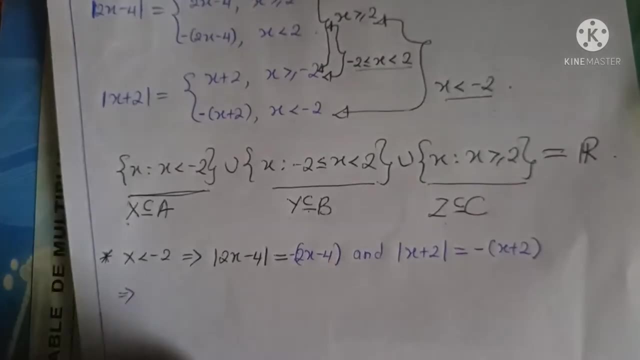 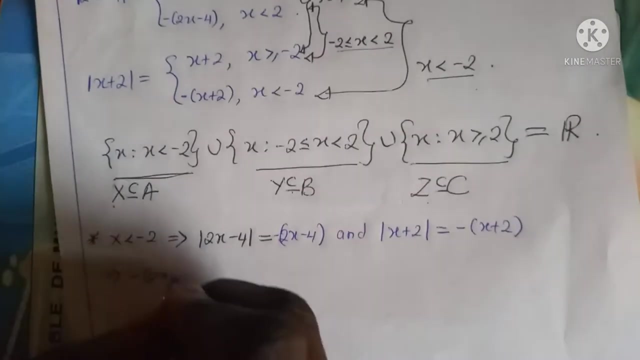 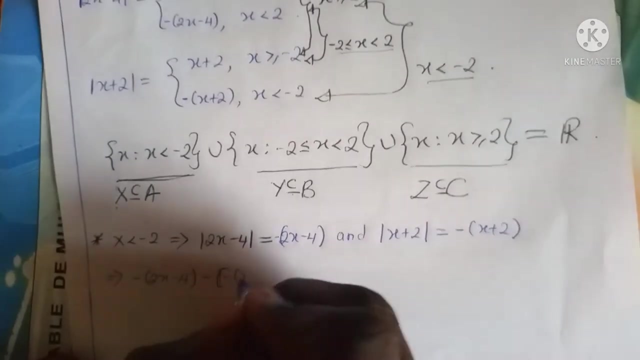 Remember, x less than negative 2 is obtained from these two branches: this branch and this branch. Okay, this will mean that from this in-equation we are going to obtain negative into 2x minus 4, minus negative into x plus 2, which is less than 6.. 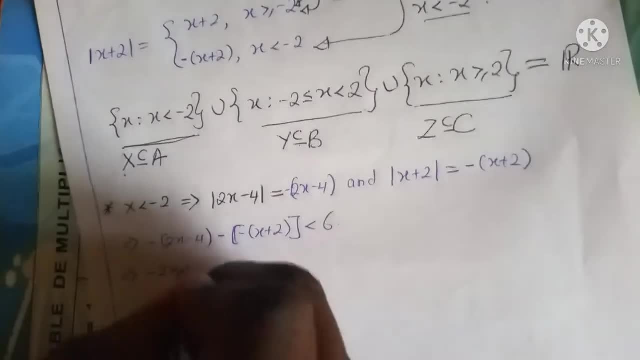 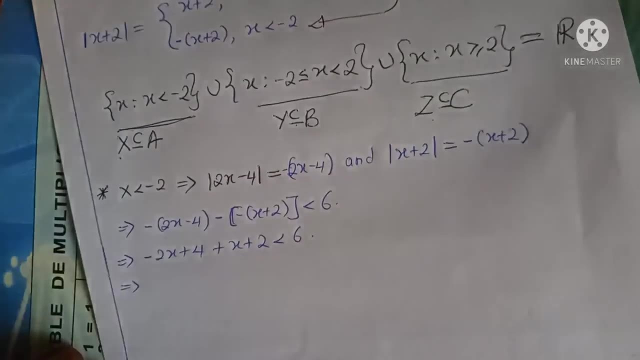 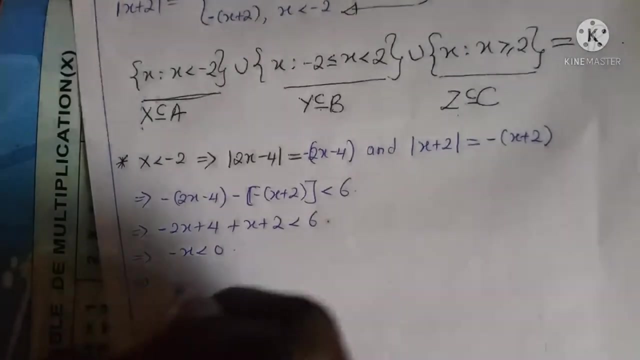 So this implies that negative 2x plus 4 plus x, x plus 2 will be less than 6.. And if you simplify this, you are going to obtain negative x, which is less than 0.. And if you divide both sides by negative 1, we are going to have x which is greater than 0. 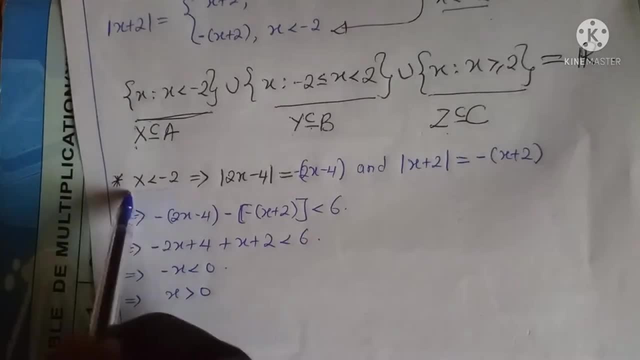 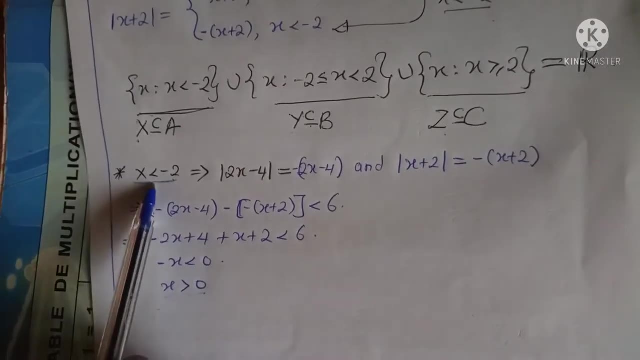 Now we are working in the set A, in this interval, And this is what we have obtained. So at this level, we must find the intersection of this and this And, clearly, if you use this interval, you will find that this is the intersection of this and this. 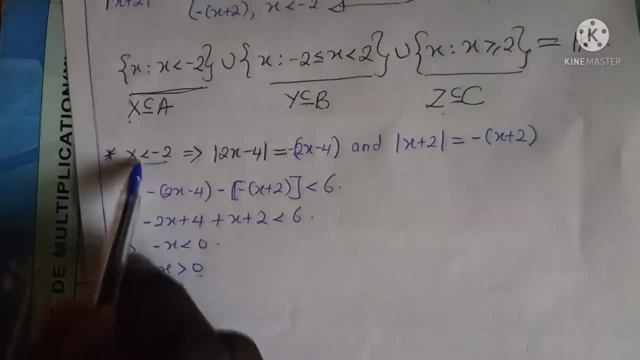 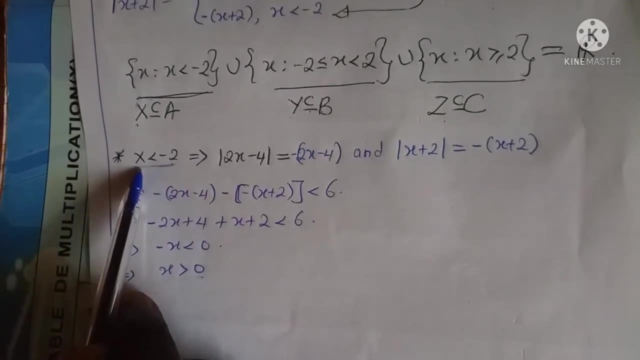 If you use a normal line, you will see that the intersection is an empty set. There is no intersection between these two intervals. There's no value of x which is less than negative 2, and, at the same time, greater than 0.. 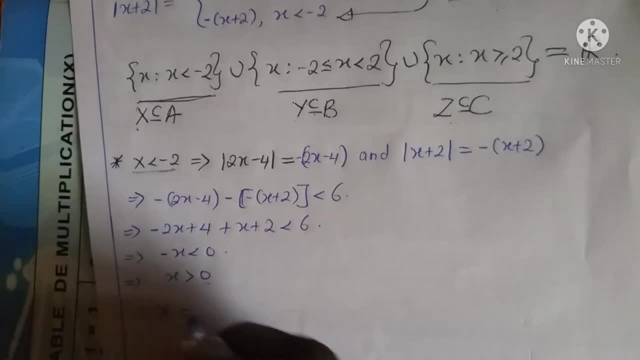 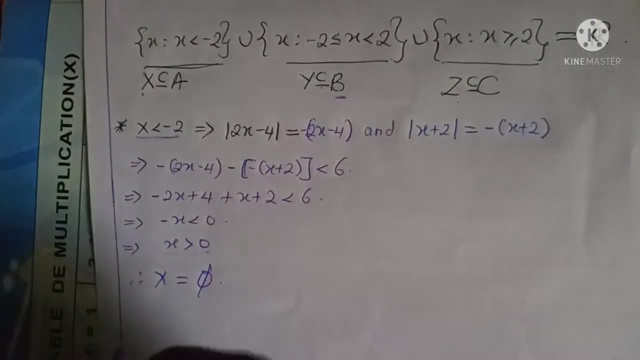 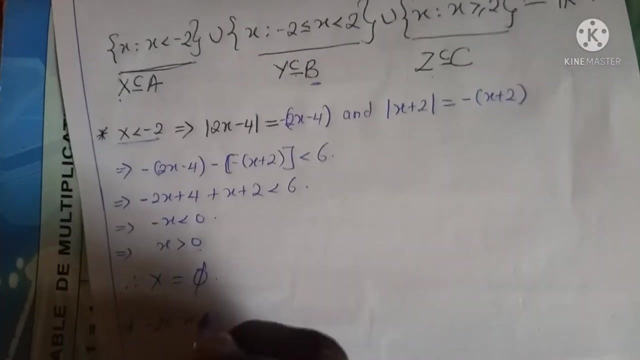 So the set x, our x here is just an empty set. We get to the set B. In B we know that negative 2 is less than or equal to x, which is less than or equal to 0. Sorry, which is strictly less than 2.. 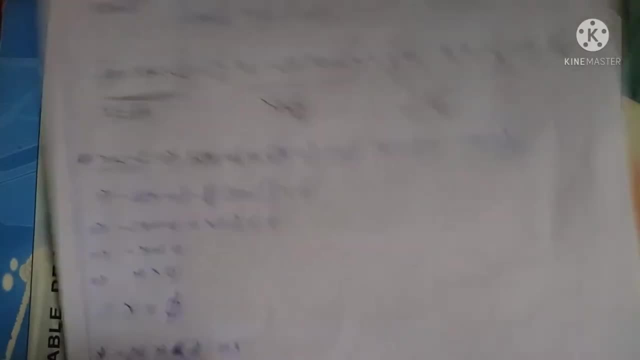 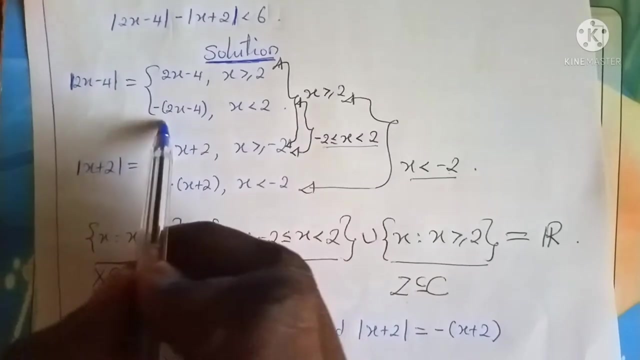 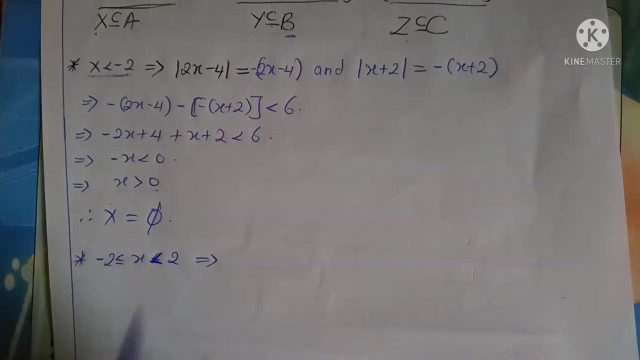 And we know that if x lies in this interval, then looking at these branches, looking at this, we know this interval is obtained from this last branch here and the first branch here. So if negative 2 is less than x, which is less than 2,. 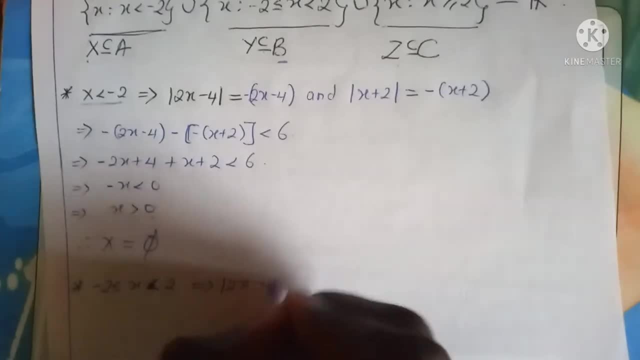 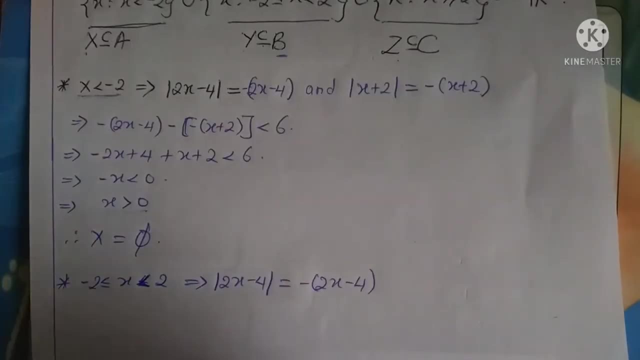 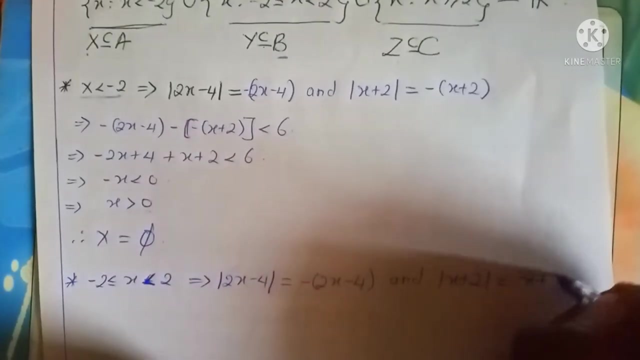 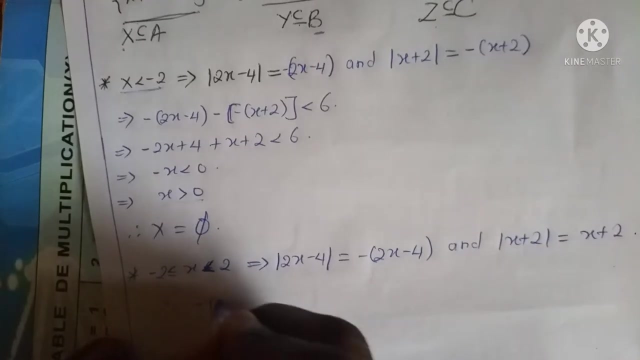 then the absolute value of 2x minus 4 will be equal to negative into 2x minus 4.. And the absolute value of x plus 2 will just be x plus 2.. Therefore, the above inequation reduces to negative into 2x minus 4, minus x plus 2,. 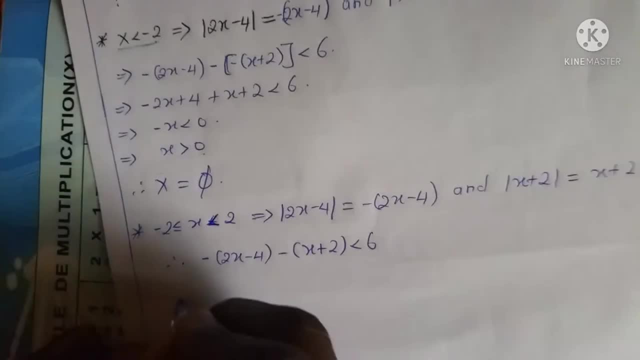 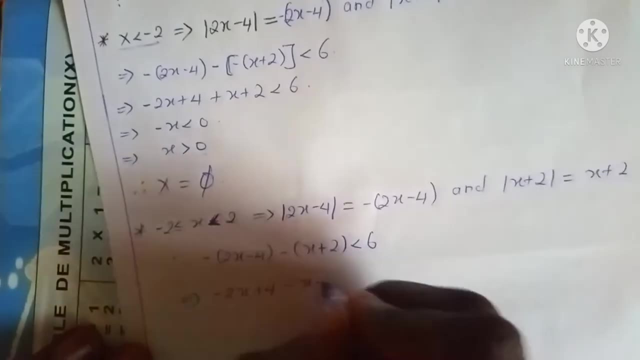 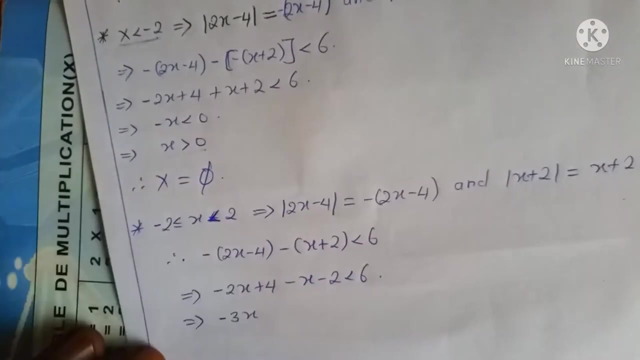 which is less than 6.. And so this implies that negative 2x plus 4, minus x minus 2 is less than 6.. And if you simplify this, we're going to obtain negative 3x, which is less than 4.. 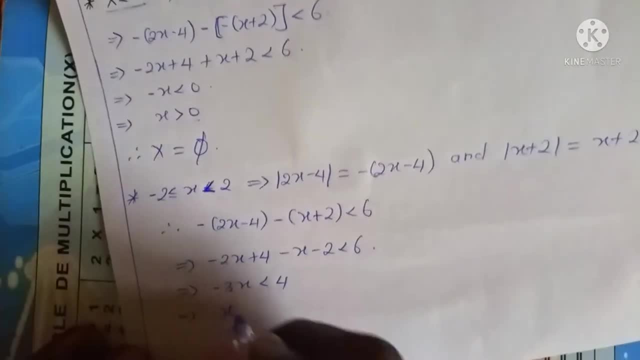 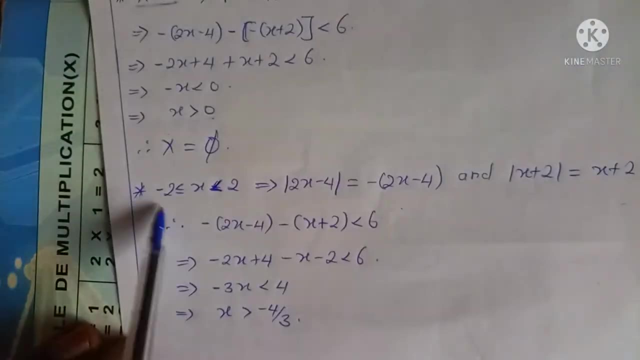 And if you divide both sides by negative 3, we're going to obtain x which is greater than negative 4 on 3.. Good, So remember, we are working in this set, So we are going to find the intersection of this. 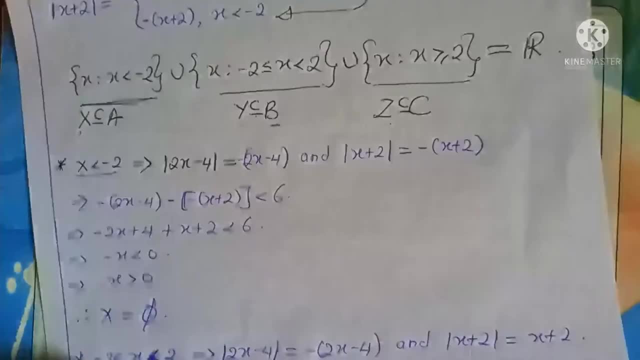 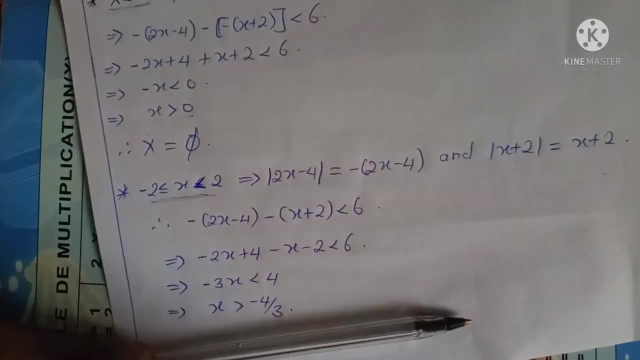 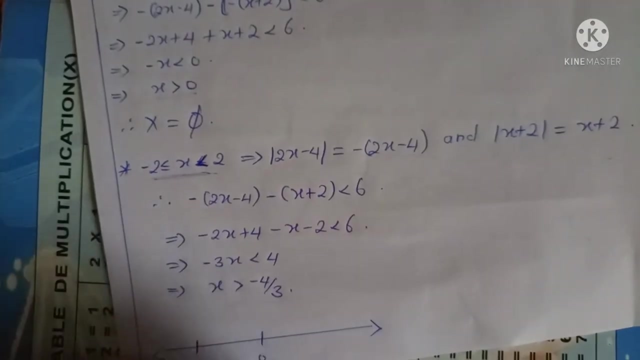 and this In order to obtain our y. Okay, good. And to do that, I will represent these two intervals on the same number line. So I'll start with the first one. So here I have negative 2. And here I have 2.. 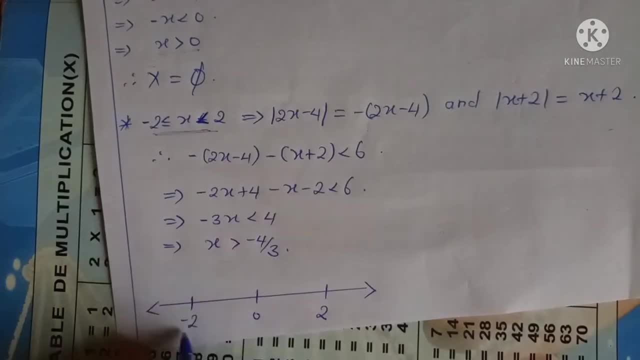 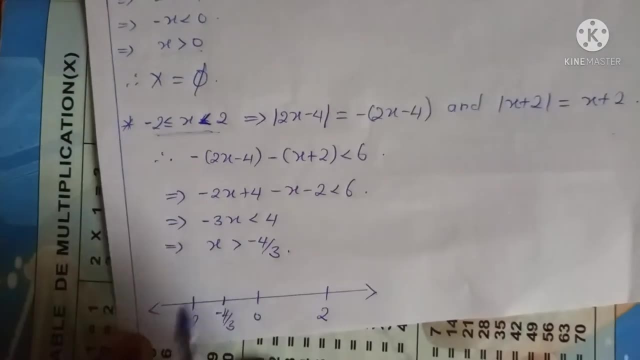 I know negative 4 on 3 is somewhere between 0 and negative 2.. So let me represent it somewhere here. And negative 4 on 3.. Good, So the first interval starts from negative 2, including negative 2,. 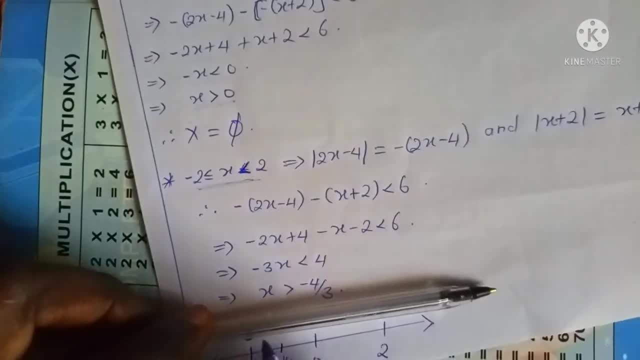 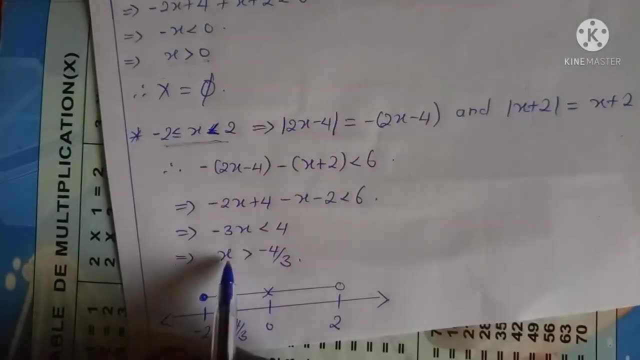 up to 2.. Excluding 2.. So that is the first interval, And the second interval is this: That is x greater than negative 4 on 3.. So it starts from negative 4 upwards. Negative 4 on 3 upwards. 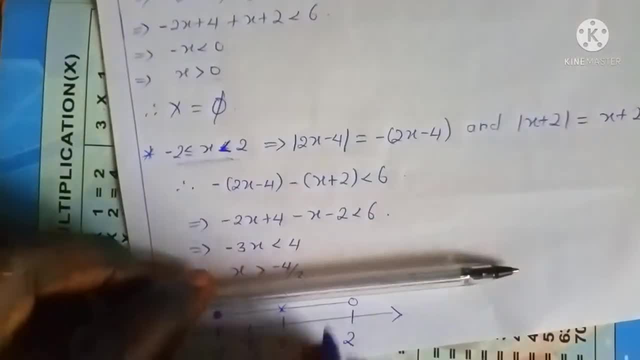 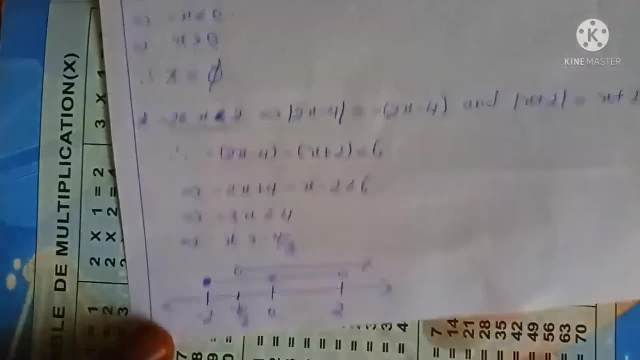 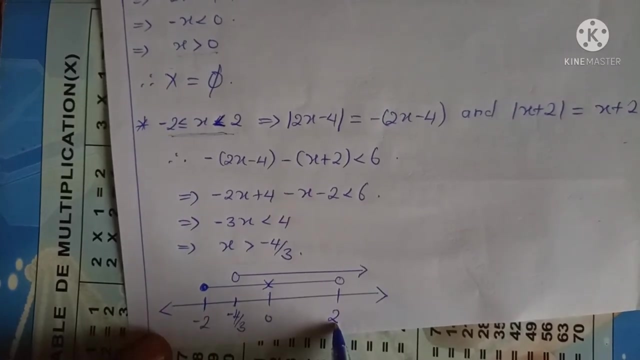 Excluding negative 4 on 3.. Good, So this is what we have, And so it shows that in this particular set, only values between negative 4 on 3 and 2 will satisfy the given-in equation. That is the intersection we have from here. 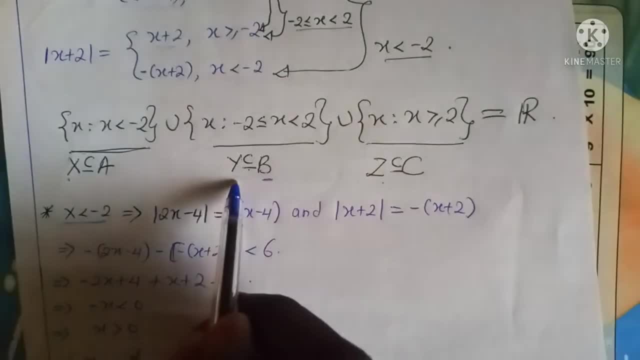 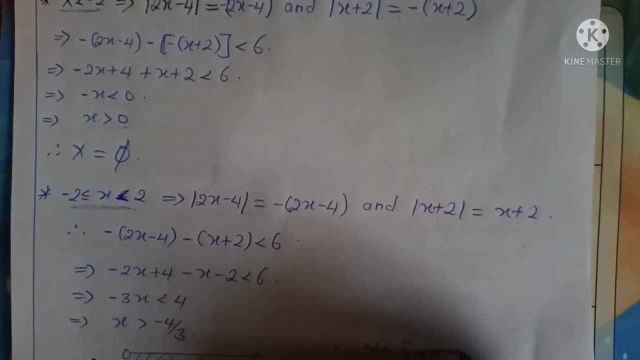 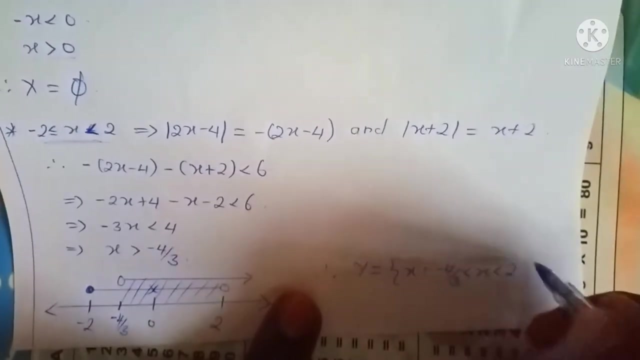 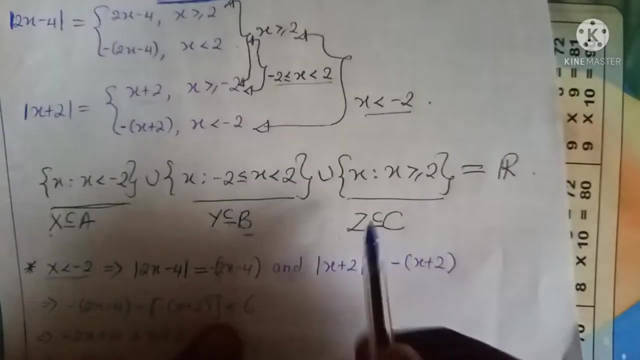 So therefore our y, that is a subset of b, is a set x, such that negative 4 on 3 is less than x, Which is less than 2.. Then we continue with z. To find z, we must start with the set c. 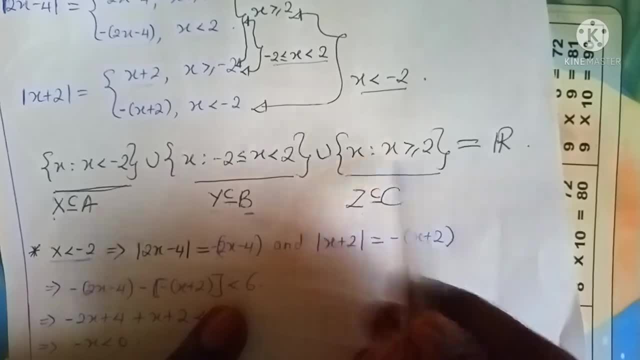 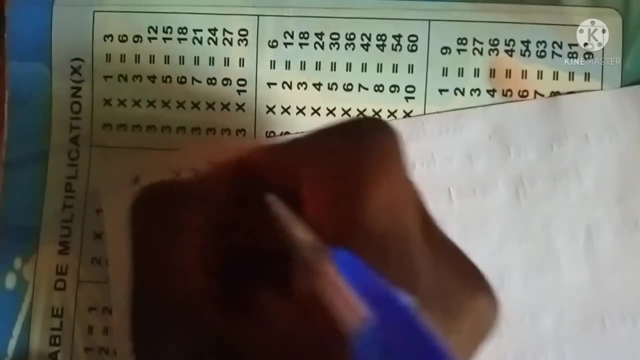 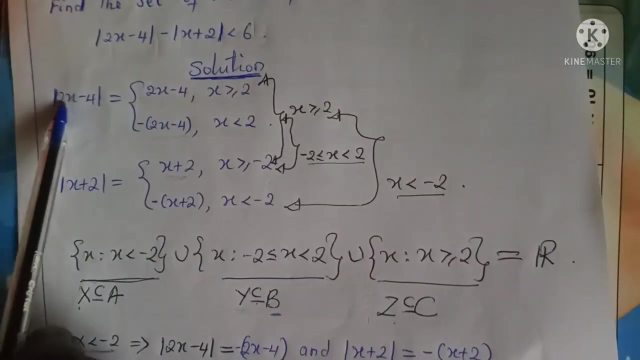 which is the interval above 2.. So we know, if x is greater than or equal to 2,, then if x is greater than or equal to 2,, then this is what we are going to obtain. The absolute value of 2 is negative 4 on 3.. 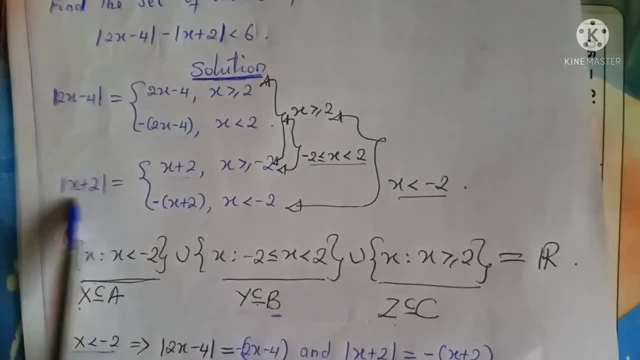 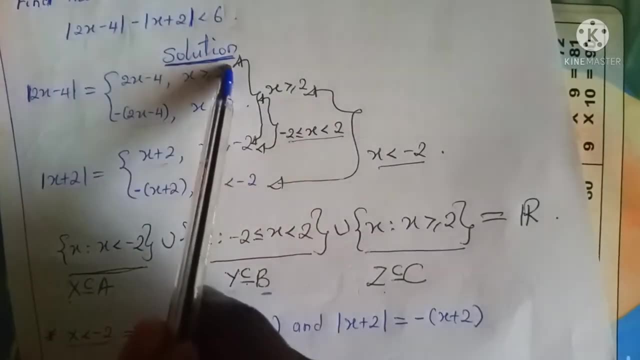 Y is equal to 2x minus 4 will just be equal to 2 x minus 4.. And then the absolute value of x plus 2 will just be equal to x plus 2.. Remember: x greater than 2 is the intersection of these two intervals here. 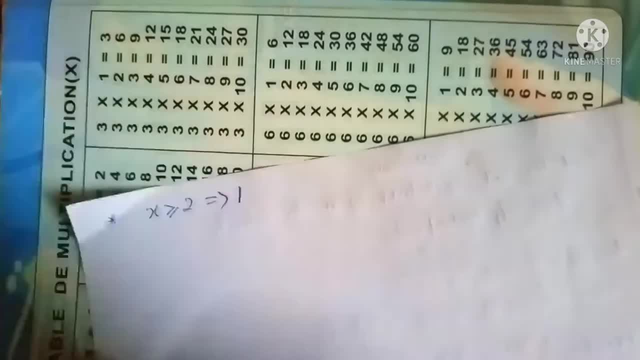 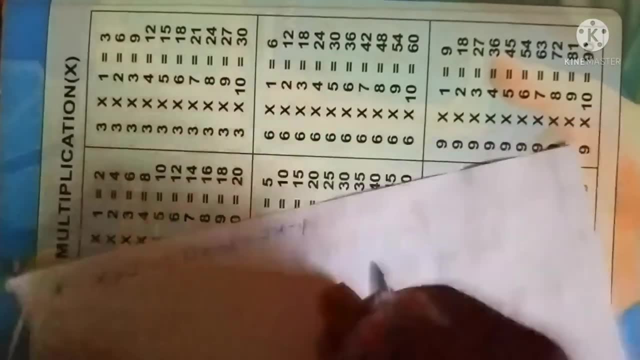 Good. So we are saying that if x is greater than or equal to 2,, then the absolute value of 2x minus 4, will just be equal to 2x minus 4.. And the absolute value of x plus 2. 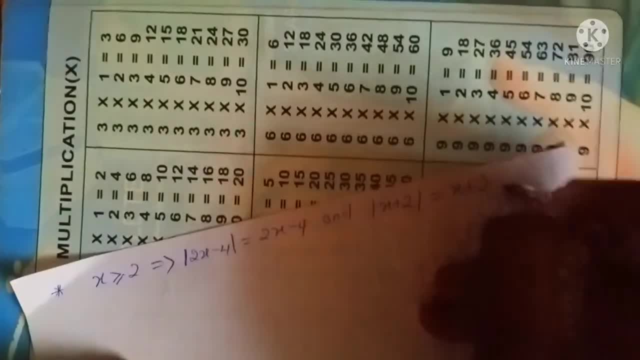 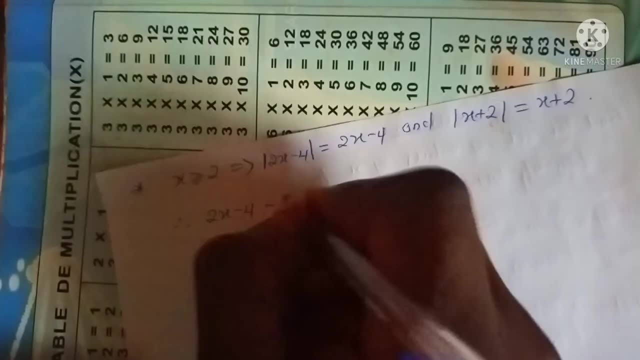 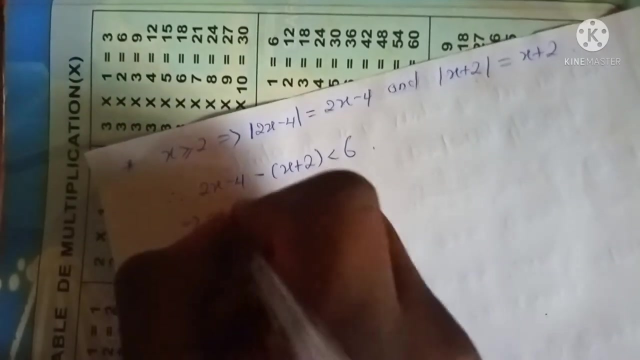 will just be equal to x plus 2. therefore, our in equation reduces to 2x minus 4 minus x plus 2, which is less than 6, and so this implies that 2x minus 4 minus x minus 2 is less than 6. 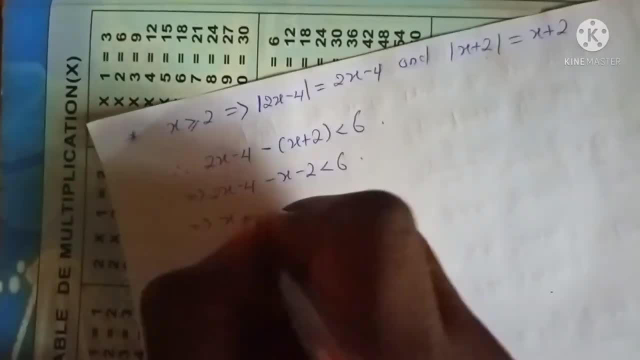 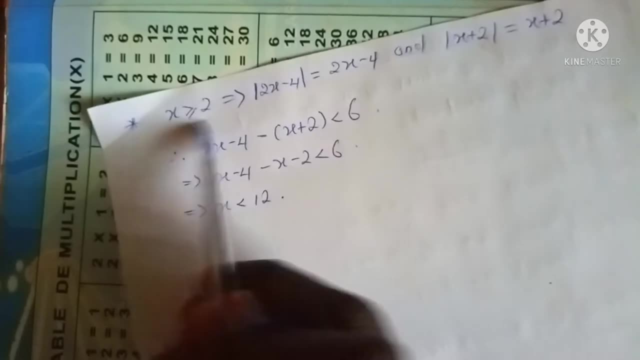 and if you simplify this, you are going to obtain x, which is less than 12. 12. good, so we are in this particular set, in this set, and this is what we have obtained. so we need to take the intersection of these two to find our z. 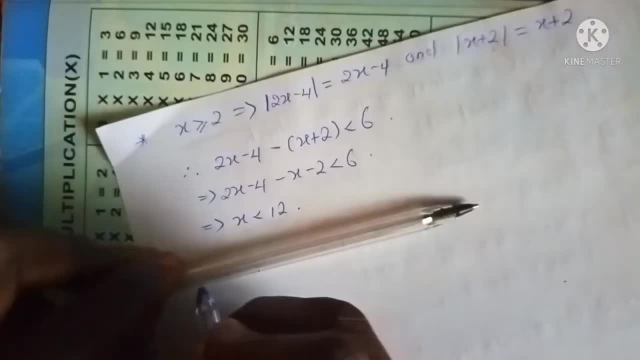 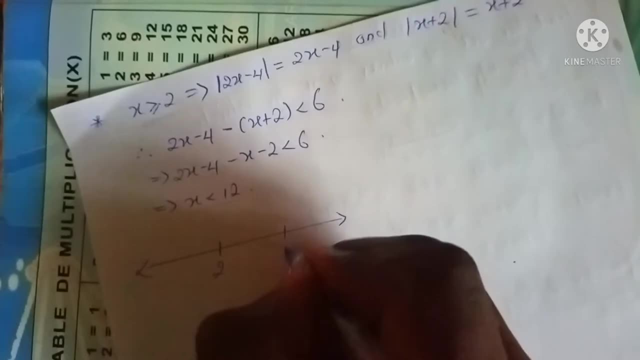 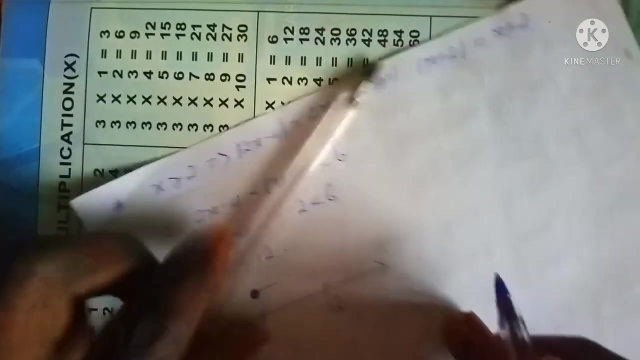 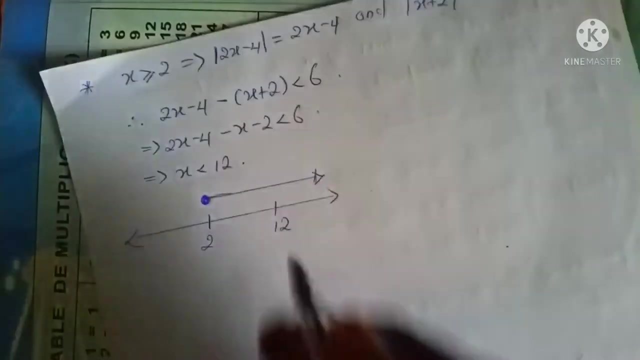 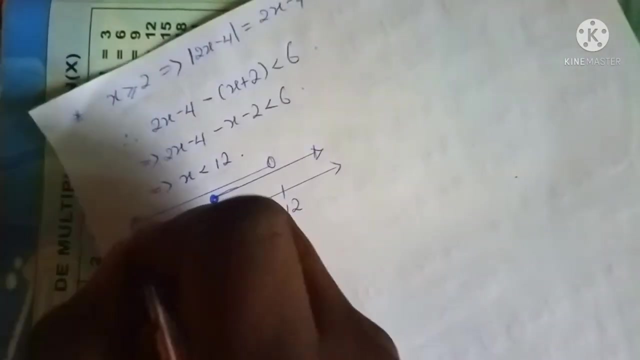 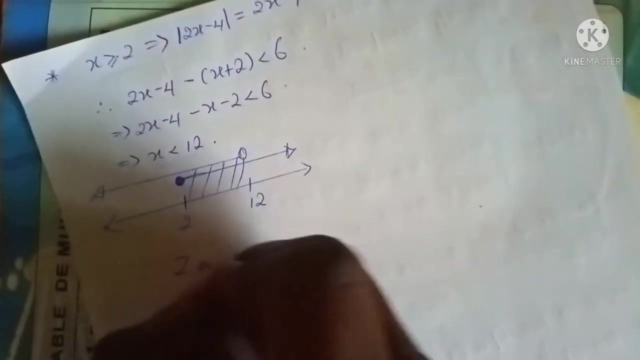 so this is 2 and here we have 12. so this is the first set x is greater than 2. so we are working in this given set and we have seen here that only values less than 12 will satisfy the above in equation. so the intersection is our z. so therefore we are saying that the set z is a set x, such that 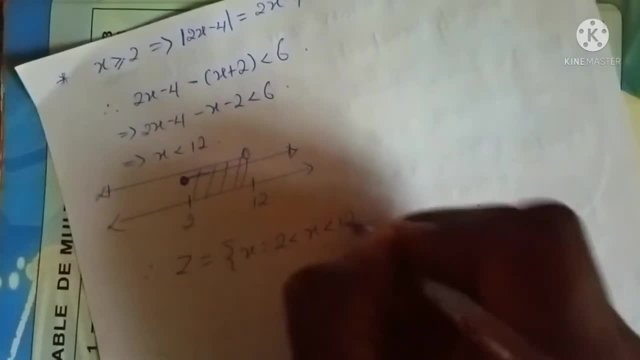 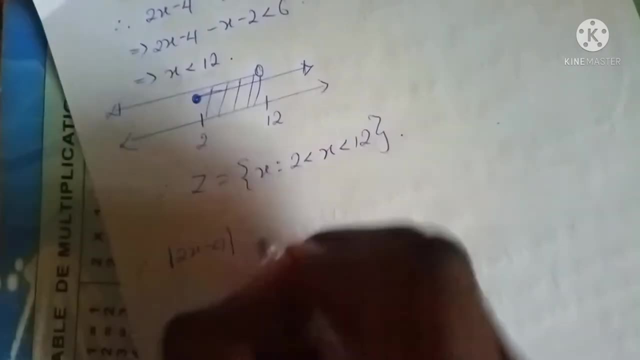 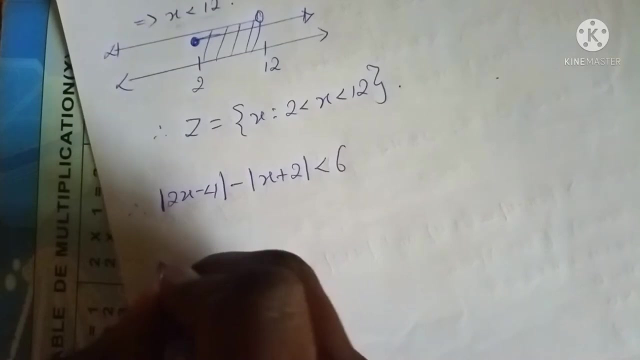 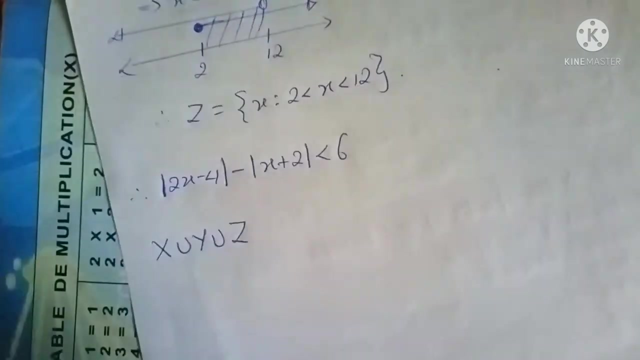 2 is less than x, which is less than 12. good, so therefore, if the absolute value of 2x minus 4, minus the absolute value of x plus 2, is less than 6, then the solution set will be given by x union y, union z, which is the set. remember our x is an empty set.